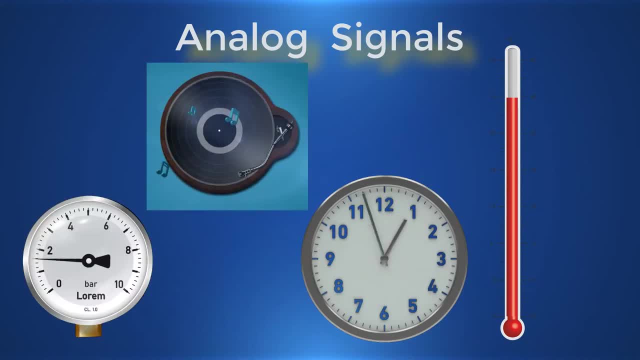 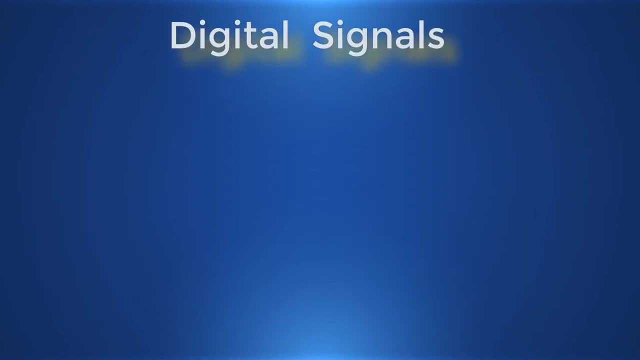 Temperature, time, pressure and sound are the examples of analog signals: Digital signals. Digital signals are signals that have only two positions, high or low, Where high is equal to 1 and low is equal to 0.. If the voltage are 2 to 5 volts, 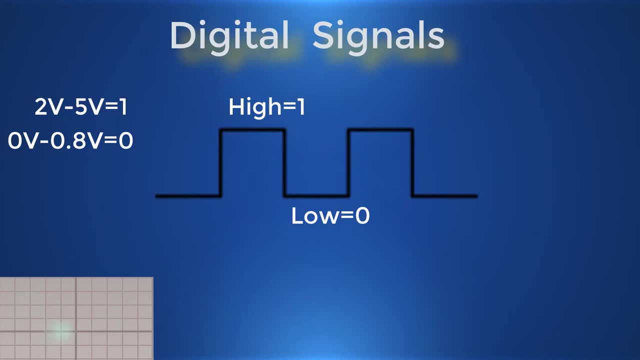 it means high or 1, and if voltage are 0 to 0.8 volt, it means low or 0. Because the position of signals in a digital system is either high or low means 1 or 0. That's why the digital signals 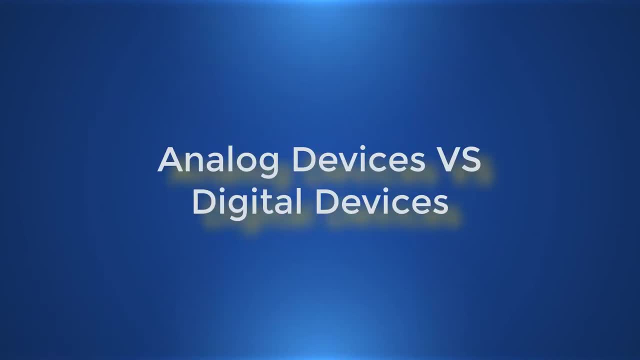 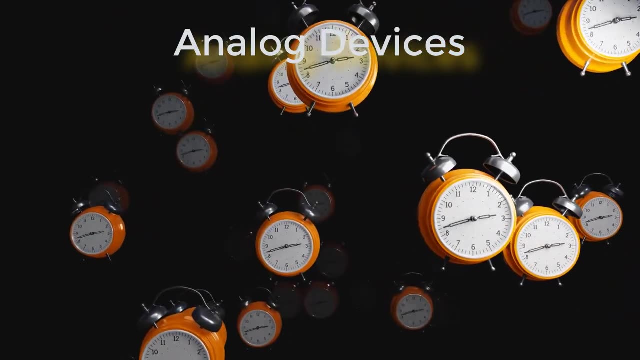 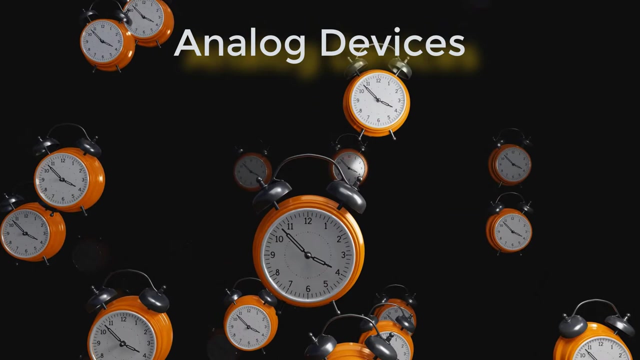 are called binary signals. also Analog devices versus digital devices. All measuring instruments that express their measured value with the help of a needle or pointer through a calibrated scale for a rating such as volt meter, ampere meter, frequency meter, temperature meter, are all analog. 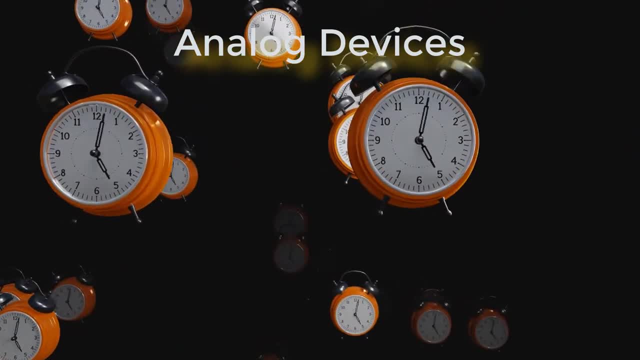 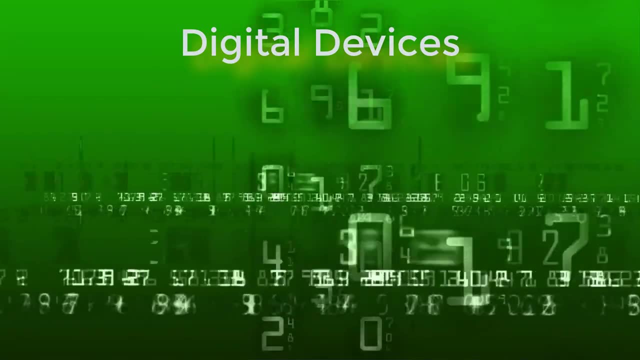 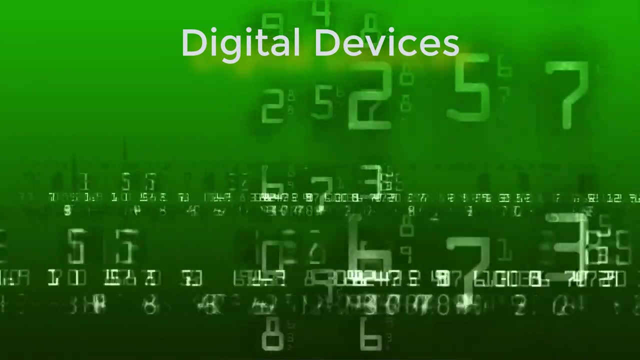 measuring instruments, because the pointers measure the value of the digital signal move constantly with changes in the amplitude of the measured values. In contrast, all measuring instruments that do not consist of pointers and scales and display their measured value in the form of individual digits or discrete digits are called digital devices, Binary codes or digital. 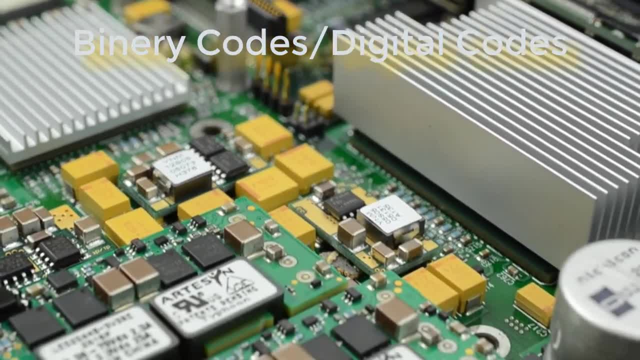 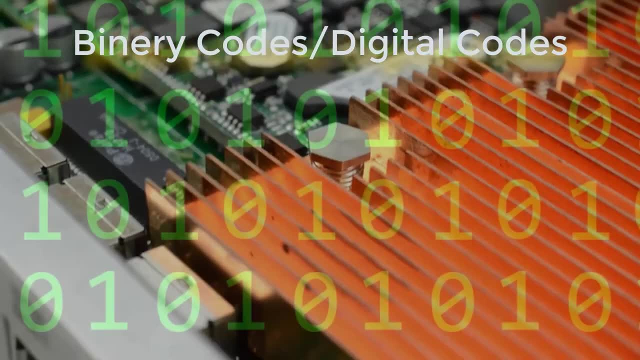 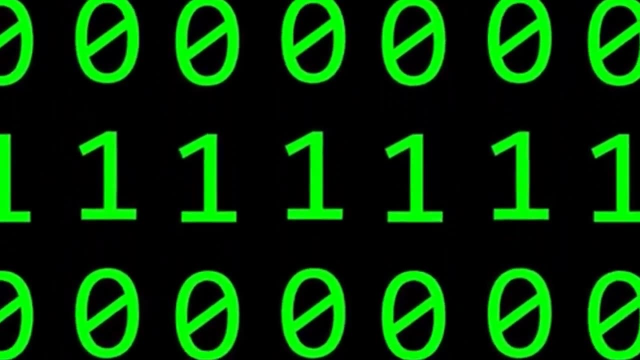 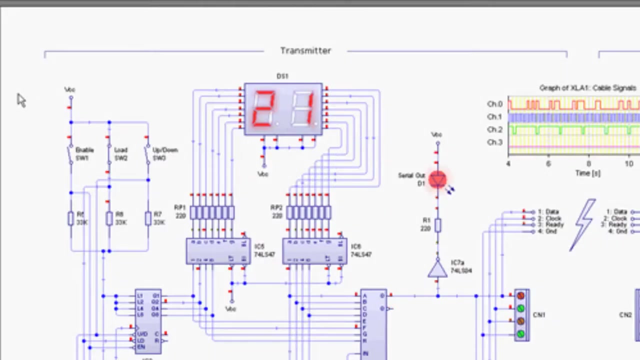 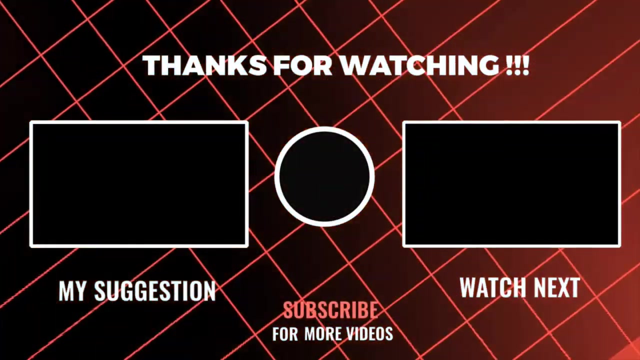 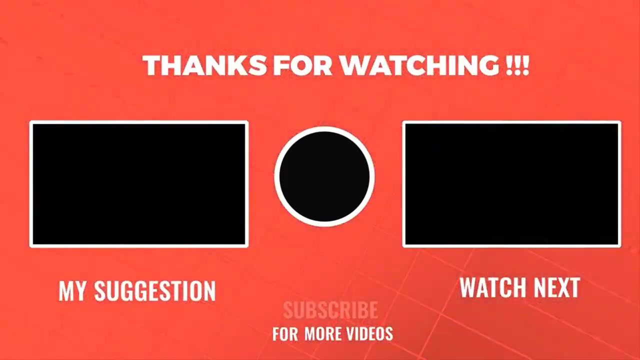 codes: Binary code Code used in digital computers based on a binary number system in which there are only two possible states. So the components or devices that process through digital codes are called digital components, and study of such components is called digital electronics. to learn more about digital electronics, please subscribe my youtube channel and press bell icon to get notification of new videos. Thanks for watching. Goodbye. Subtitles by the Amaraorg community.